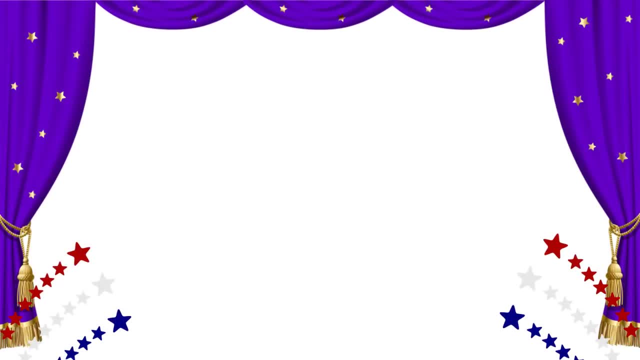 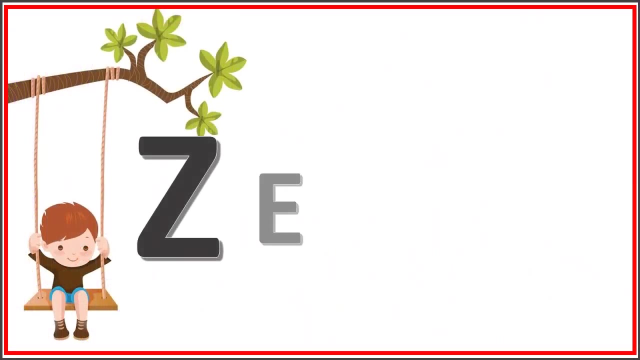 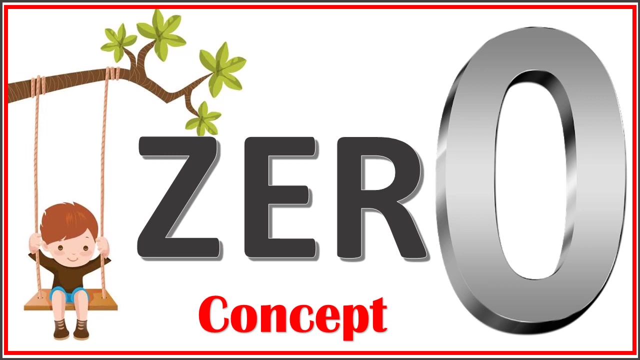 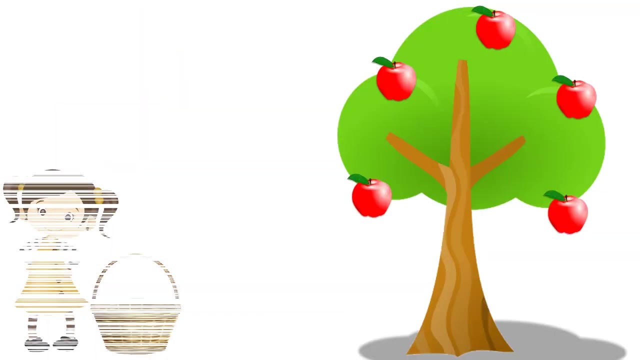 Hello kids, Today we will learn about the zero concept. Yes, let's get to know about the number zero. Come on, let's get started Now. let's try to understand the concept of zero with a little example Here, this: 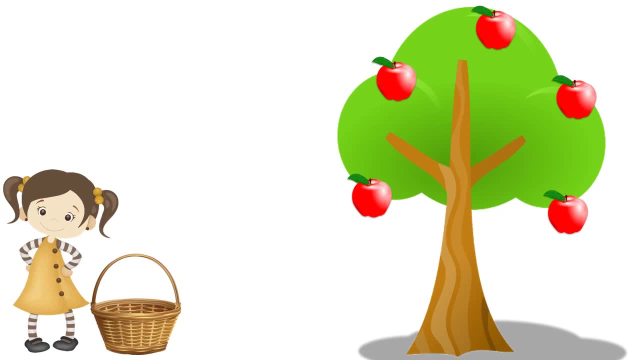 little girl wants to collect the apples from the tree. Now let's count the number of apples: 1,, 2,, 3,, 4,, 5.. So there are 5 apples on the tree. Now consider one apple falls off from the tree. So let's count the number of apples on the tree: 1,, 2,, 3,, 4.. So there, 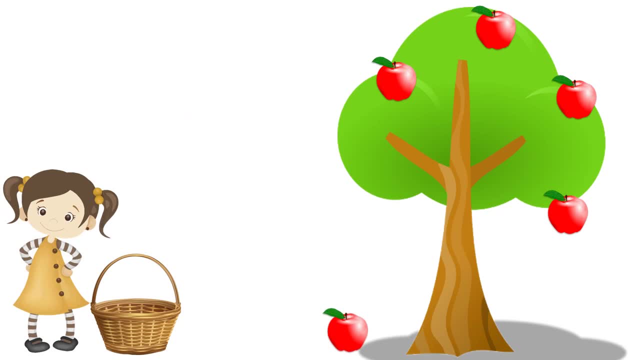 are 4 apples on the tree. Now another apple falls off from the tree. Now let's count again. Now, another apple falls off from the tree. Now let's count the number of apples on the tree: 1,, 2.. So there are 2 apples on the tree. Now one more apple falls off from the tree. 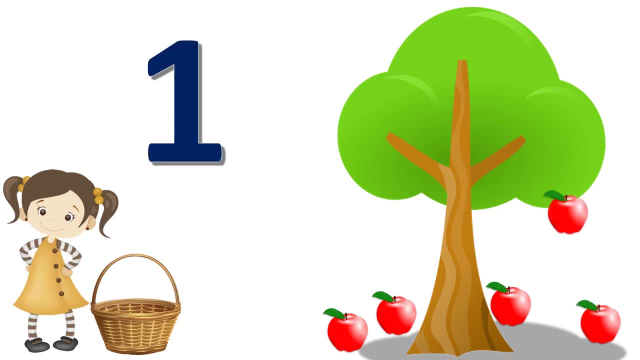 So we have 1.. So one apple is on the tree. Now this apple also falls off from the tree, So can you see any apple on the tree? Yes, there are no apples on the tree, So it is said to be zero. 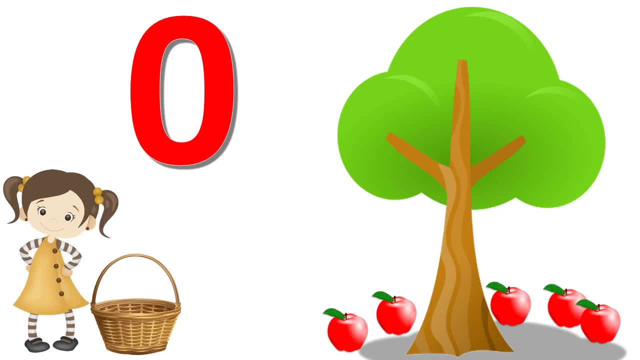 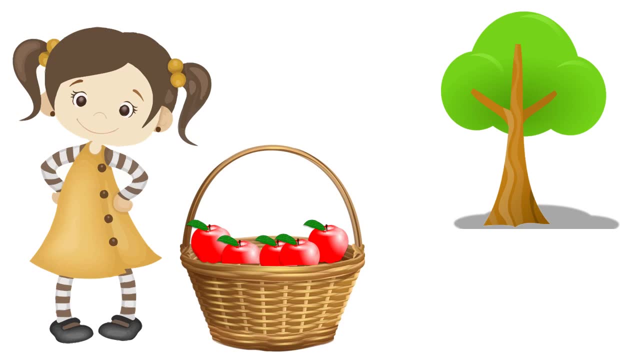 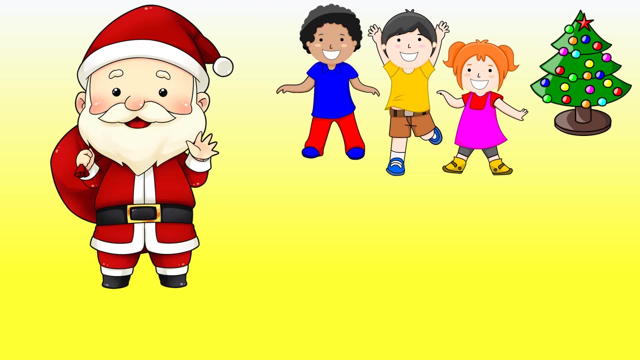 So there are zero apples on the tree. Now this little girl has collected all the apples from the tree. So there are zero apples on the tree Now. let's take another example. Here we have the Christmas celebration And the Santa wants to give some gifts to the little ones. 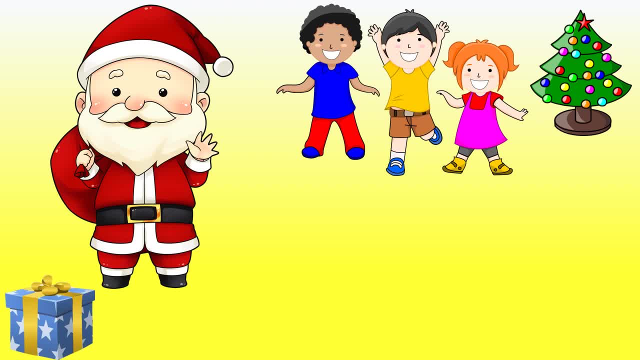 Now let's count the number of gifts: One, two, three. So there are totally three gifts with the Santa. Now the Santa shares one gift to the little one. Now let's check out the number of gifts left out with the Santa. 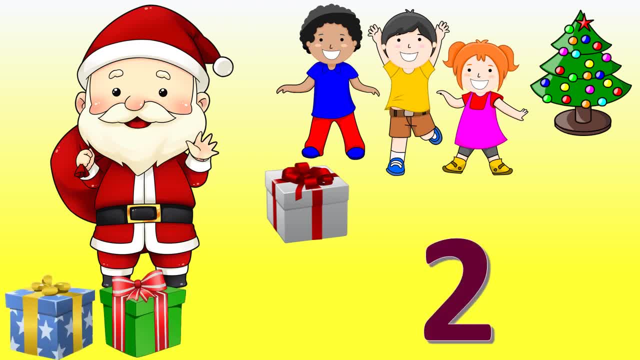 One, two. So there are two gifts left with the Santa. Now, here the Santa shares another gift to the another kid, So the number of gifts left with the Santa is one. So there is one gift box left out. 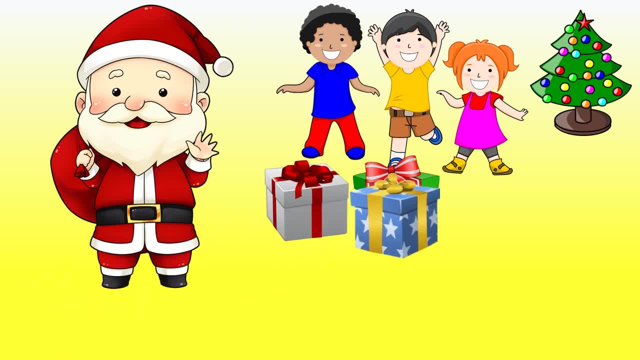 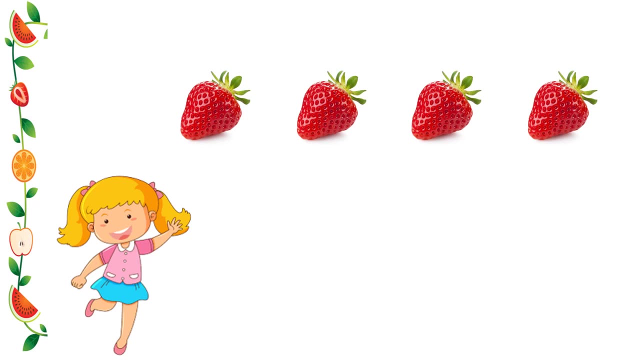 Now the Santa shares the last gift box to the little one, So there are zero gifts left with the Santa. So here we say it as zero. Now let's take another example. Now let's understand the concept of zero with another example. 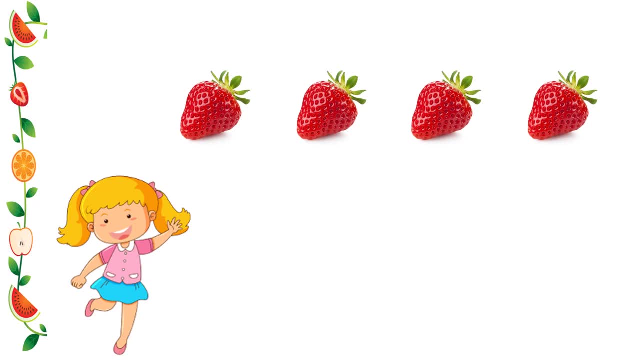 Here we have a little kid. She loves strawberries. Now let's count the number of strawberries: One, two, three, four. So we have four strawberries. Now, here, the little one ate one of the strawberry. So now let's count the number of gifts left out with the Santa. 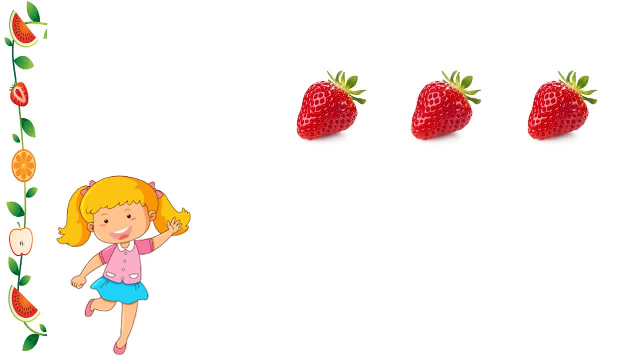 One, two, three. So there are three strawberries left out. Now this little ate another strawberry. Now let's count the number of strawberries left out: One, two, So there are two strawberries left out. The little one ate one more strawberry. 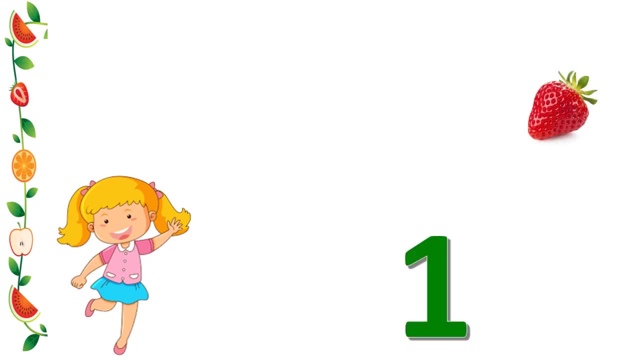 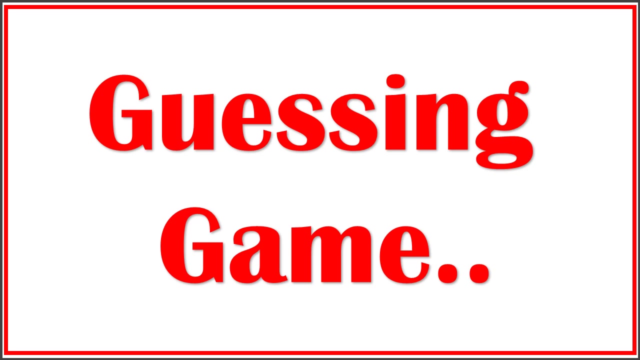 So we have strawberry left out. The little one ate this strawberry also, So there are zero strawberries left out with her. So this is the zero concept. Now let's play a guessing game. I'll be showing you a set of pictures and you have to find out. 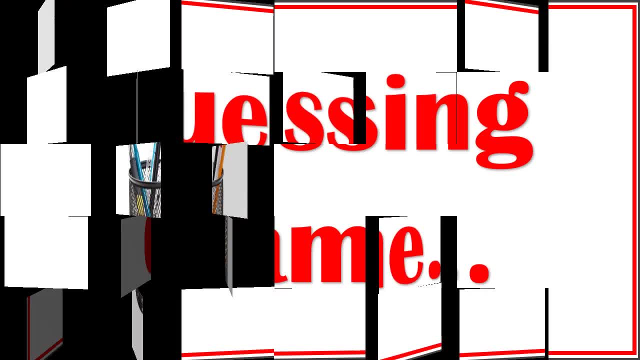 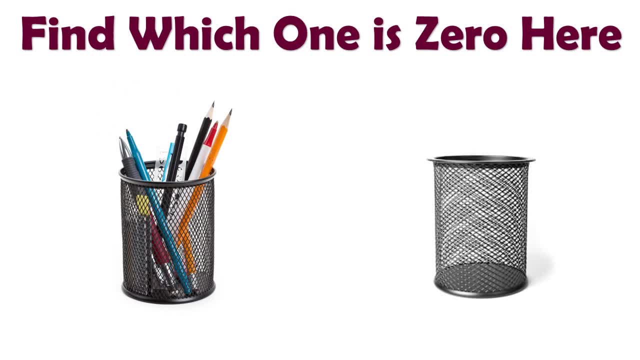 which one shows zero. Here I have two pen stands In this. you have to find which one shows zero. Yes, the second pen stand shows zero. The first pen stand has a set of pen and pencil. I hope you enjoyed this video. If you liked it, please subscribe to my channel.